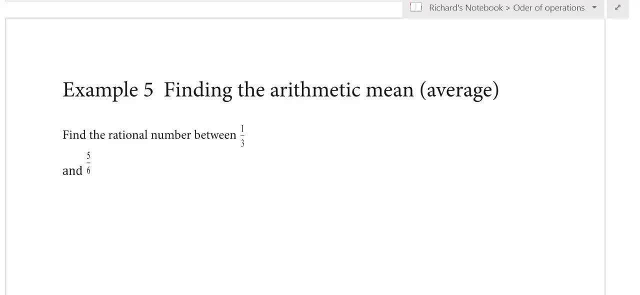 Example 5, finding the arithmetic mean or the average. Well, say you have two rational numbers, 1, 3rd and 5- 6th. You want to find the arithmetic mean of those two numbers, the average. Well, how do you find an average? Well, let's suppose we've got some easier numbers like 2 and 4.. 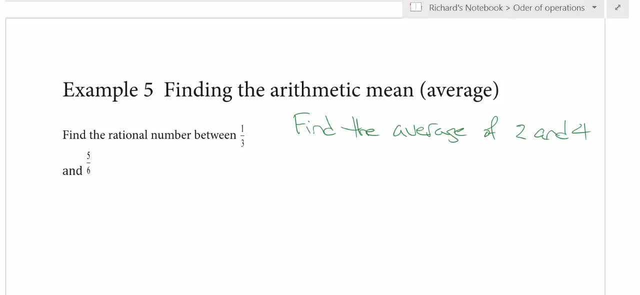 So we want to find the average of 2 and 4.. Well, what do we do? Well, you would take 2 plus 4, and you would add the two numbers together to get 6.. And that's the sum of the two numbers. Then you would take 6 divided by 2, because there are two items. 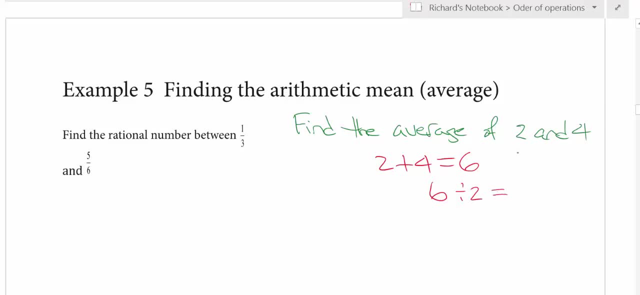 and you would get the arithmetic mean, Or in other words the average, which is 3.. I can do the same thing with these fractions. I'm going to add 1- 3rd and 5- 6th, and then divide by 2 to get the mean. 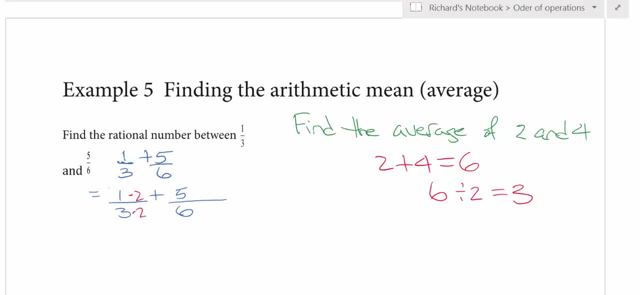 So I've got to get a common denominator. Well, really, if I multiply 3 by 2, that'll give me 6 for the denominator. That's the common denominator for the first fraction, And that's what I'm going to do. And what I do to the bottom, I do to the top. 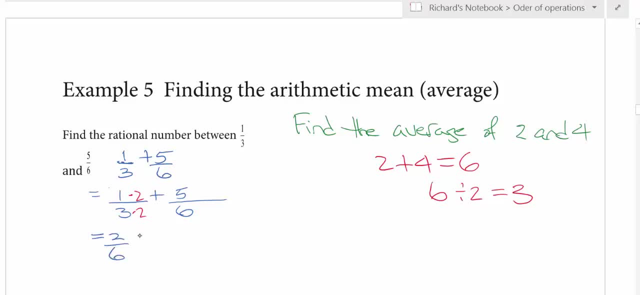 So I'm going to have 2, 6 plus 5. 6 equals 7 over 6.. So now I've got to divide 7 over 6 by 2.. So here we go: 7 over 6 divided by 2.. Well, dividing by 2 is really the same as 2 over 1.. 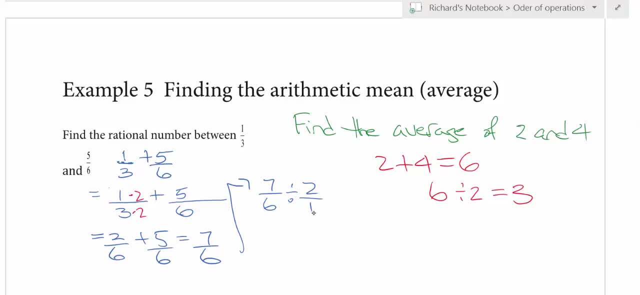 So I'm going to take the second fraction. I'm going to swap the numerator with the denominator, So this will be equal to 7 over 6 times 1 over 2.. Which equals 7 times 1 is 7.. 6 times 2 is 12.. 7- 12ths. 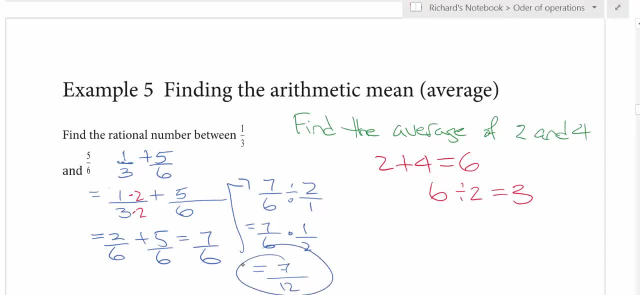 So 7 12ths is the arithmetic mean of 1, 3rd and 5 6ths.